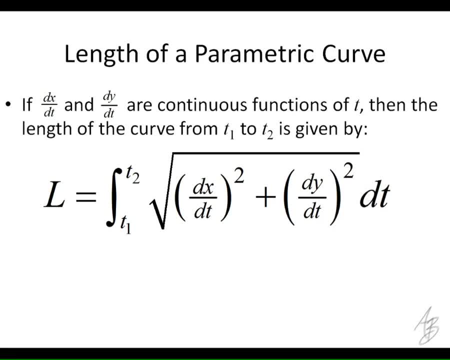 And then the square root of that is basically the distance formula. So to me this formula is actually easier to remember than that other one, because it makes more sense relative to other things that we did. So we're going to integrate from our starting time value to our ending time value of the square root of dx- dt squared plus dy- dt squared. 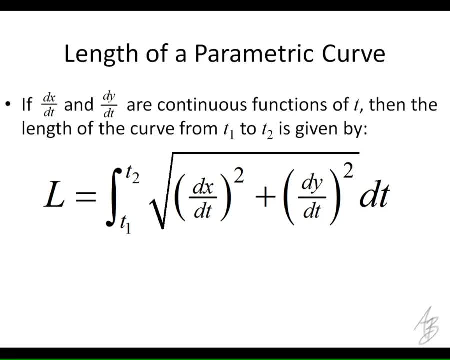 which is the distance formula With respect to time, and that's going to give us the length of the curve. Or another way to interpret this is distance traveled. So if you're traveling along a parametric curve, this tells you how far you traveled, because that's the length of the curve. 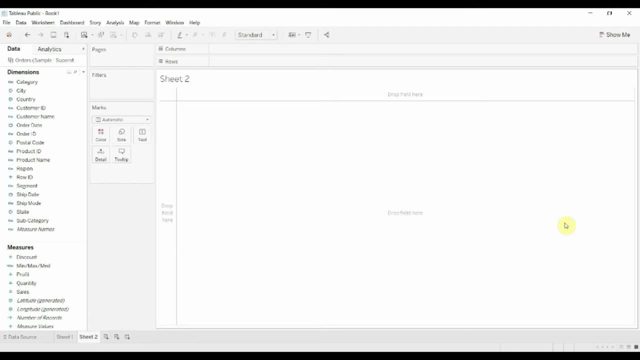 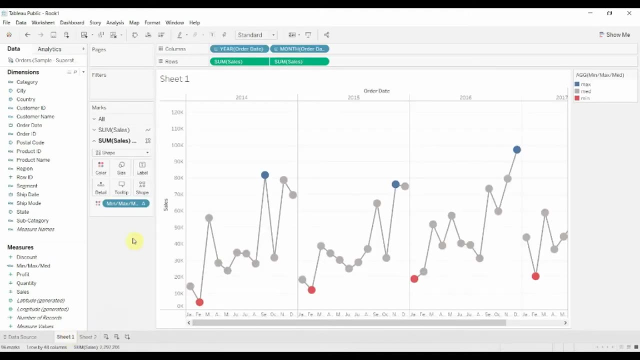 Hi folks, and welcome to another episode of Tableau in Two Minutes. Today we're going to walk through how to highlight the minimum and maximum values in a bar chart. If you watched the previous video, you may have seen how we did this for a line chart and it was a little bit complicated. 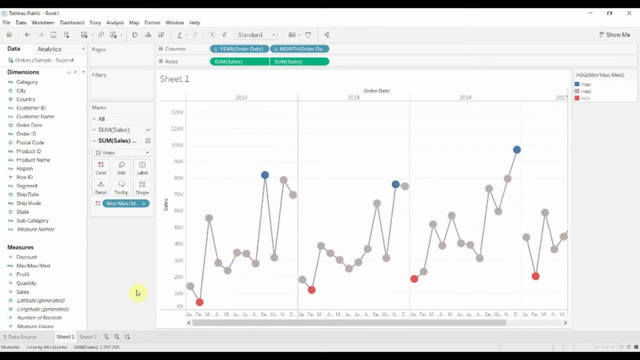 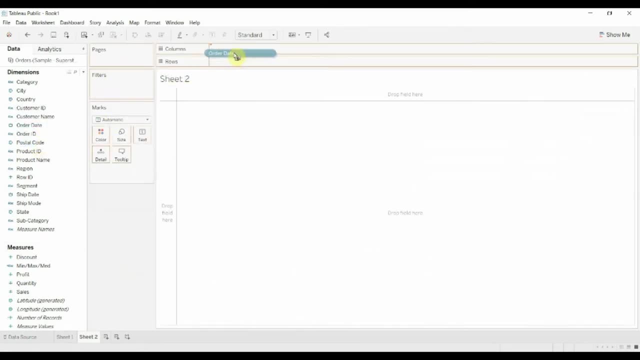 We had to do some funky stuff with some dual axes and create a table, calculation and all that sort of fun stuff. But to do it with a line chart, fortunately, is a little bit easier. So we're going to go ahead and drag order date out onto our columns shelf here. get rid of quarter. 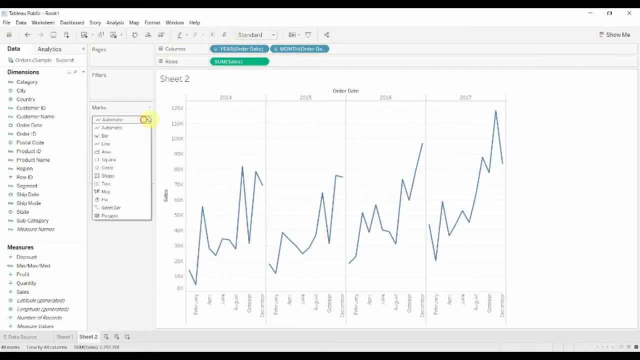 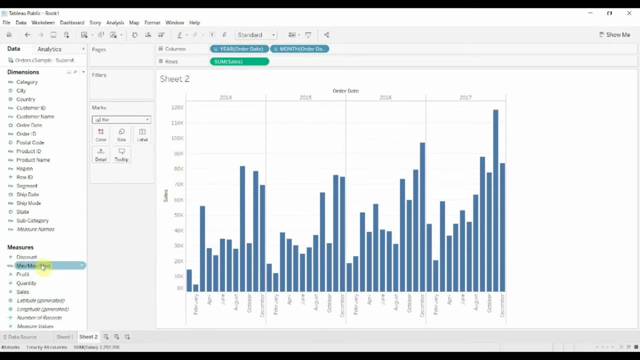 And then we're going to take sales, drag sales out onto the row shelf, And then we're going to go ahead and set this to be a bar chart instead of a line chart. Now, because we have this set as a bar chart, we can take our min, max and medium. 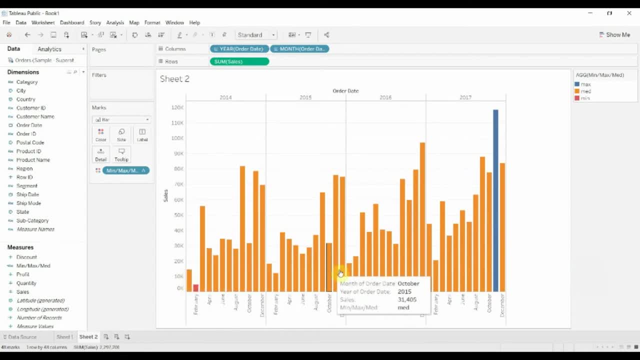 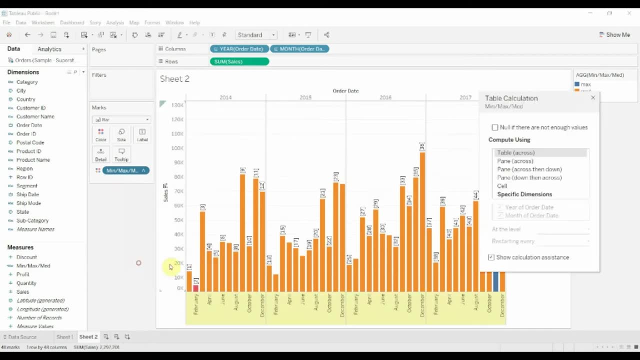 And you can see already that we've gone ahead and the colors have already been set for us, based on the maximum and based on the minimum. But let's go ahead, Edit this as we did before. We're just going to compute this within each year.